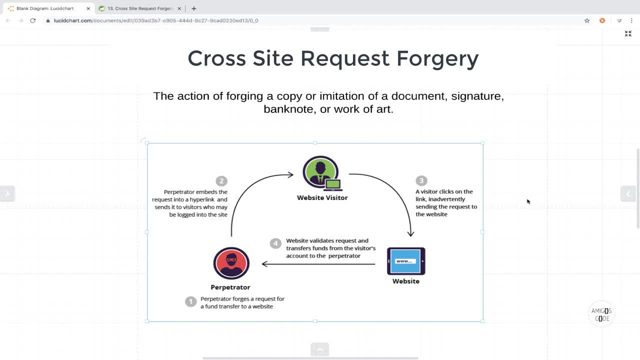 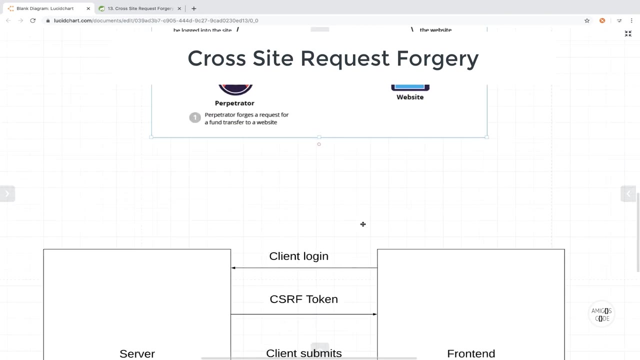 Details. So the way that spring security protects us from this kind of attack is by enabling cross site request forgery, which we have disabled right here. So when it's enabled, what happens is this: So the front end right. So this is the client, right. 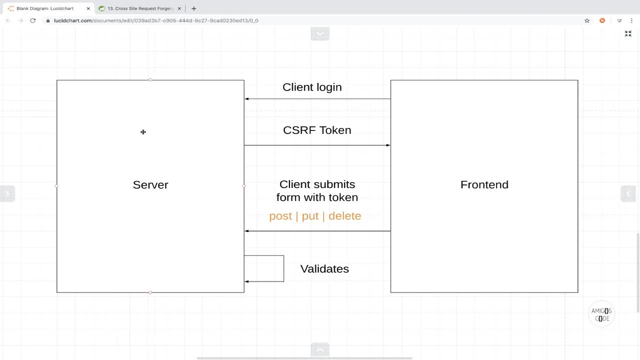 So the client? So when the client logs in into our server, spring security sends a cross site request forgery token into a cookie and then the front end uses that token for any form submission. So form submissions usually are post put or delete. 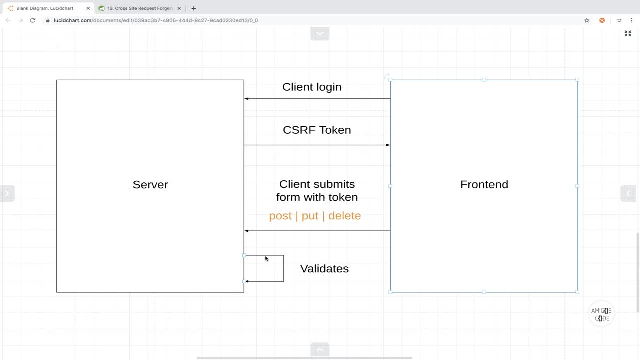 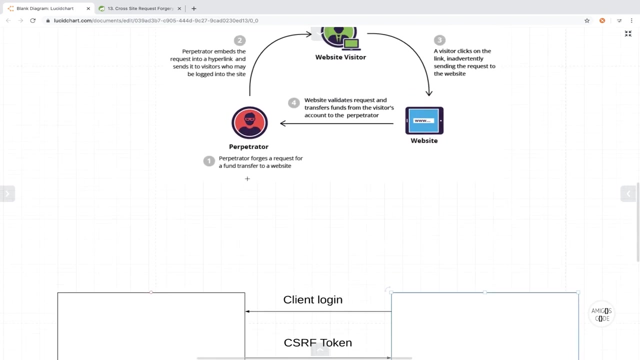 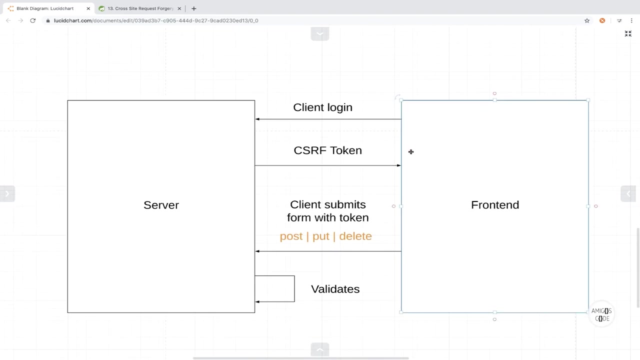 And then the server validates that token to see whether it matches what the token is The server had sent previously. So when CSRF token is enabled, there is no way for this attacker right here to know what was the original token that the server had generated for a particular client. 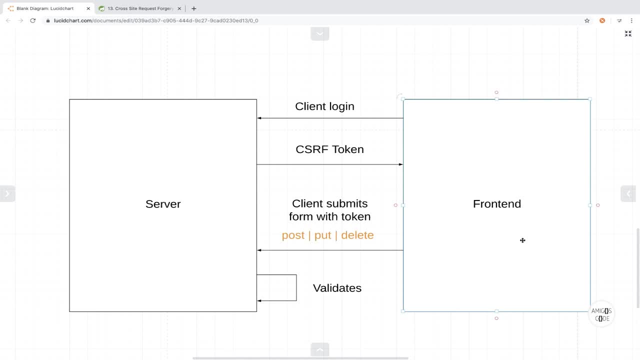 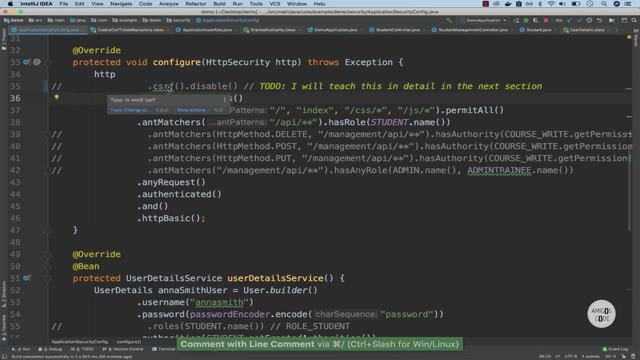 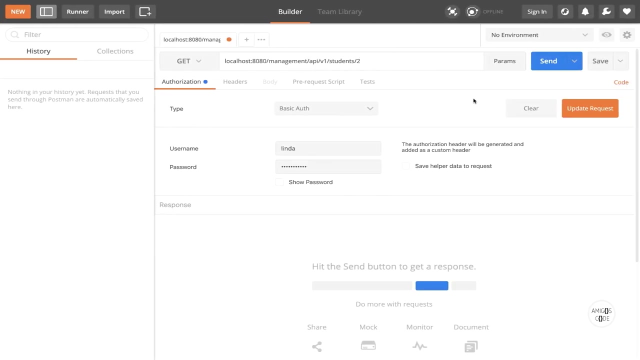 And with this problem solved. So let me go back to IntelliJ. and right here. So let's comment this line out. right? So we're going to enable cross site request forgery. So if I restart the server, there we go. And if I open a postman, so right here. 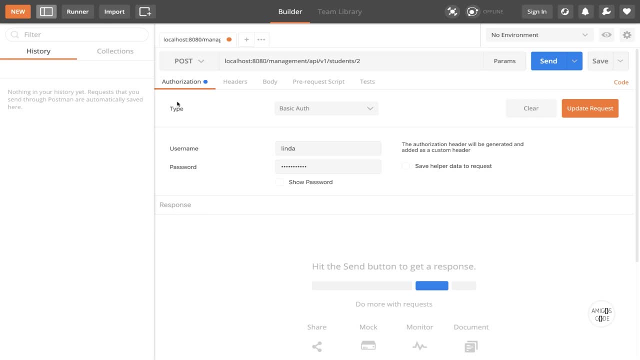 So remember before Linda was able to post requests. So if I now try and let's actually first send a get request, So let's send a get request, There we go, So you can see that this works. But now, if I go ahead and send a post request and inside 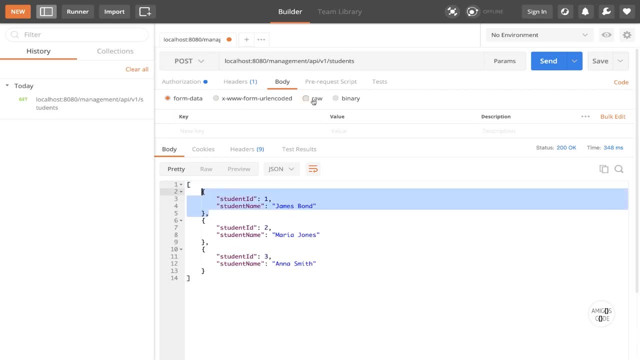 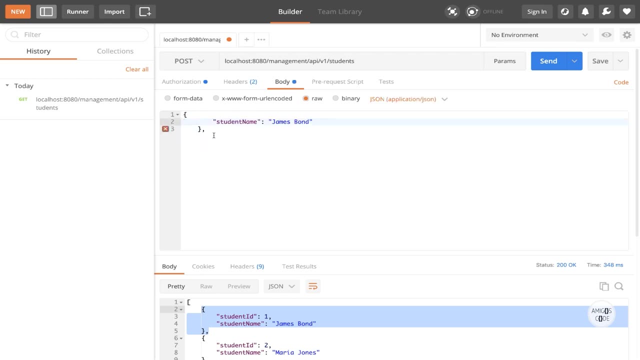 of the body. So let me actually grab this student and this will be raw. and then Jason right here, So that will be empty. So if I now try and send this payload right here, So I'm going to send this payload. You can see that, Linda, she's forbidden from performing this. 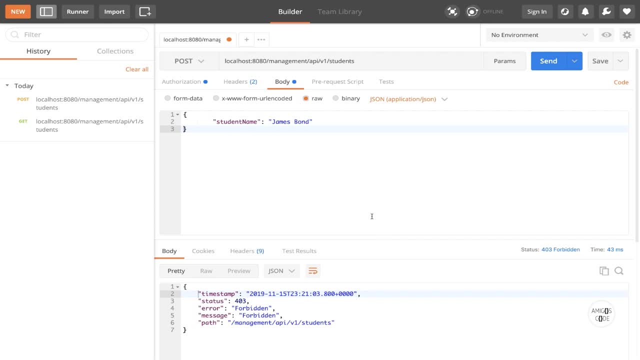 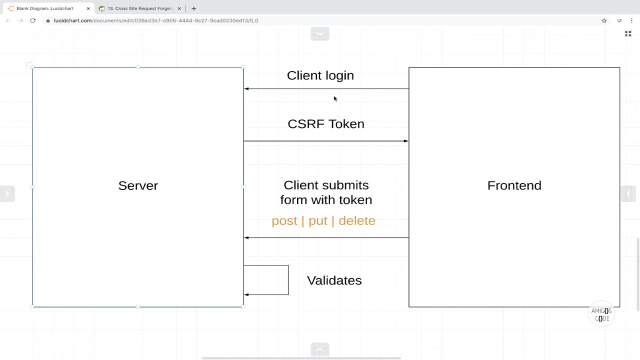 request. So spring boot security Is doing its work. So basically, so right here. So the client is logged in with basic auth, Then the server sends the actual CSRF token, right? So we actually haven't got this part yet. I'm going to show you exactly how to do it. 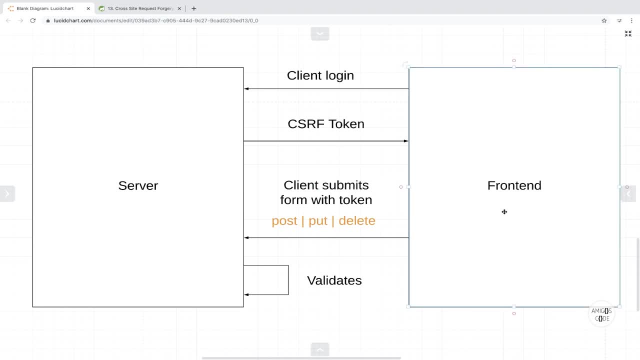 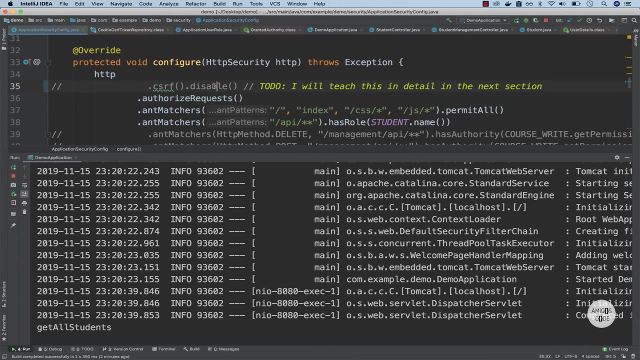 But now, when the front end sends the actual form I post or delete, this bit kicks in. So the validation kicks in And because we haven't sent any token, the request is rejected. So if I go back to IntelliJ and let me comment this again, 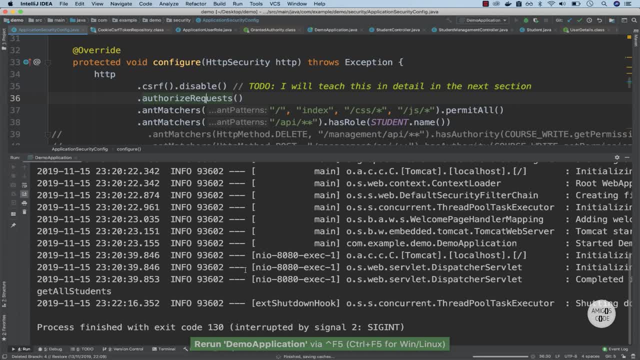 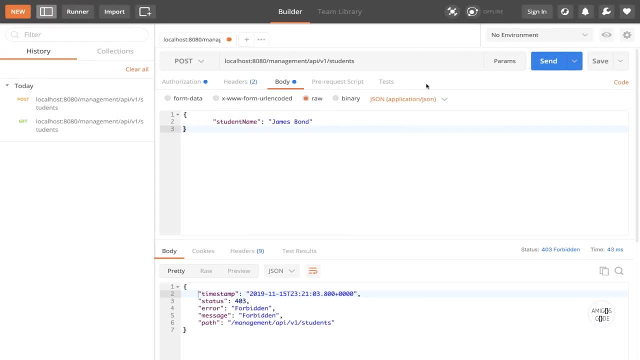 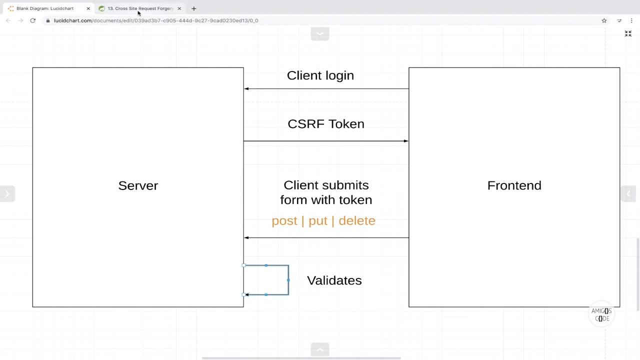 and restart the server. there we go Now. if I send the request again, you can see that now we get a status code of 200.. Now it works. So when should you enable cross site request for? So on the actual official documentation, it says that the recommendation 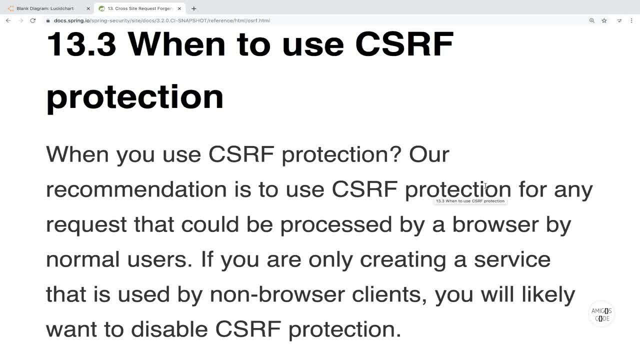 is to use CSRF protection for any request that could be processed by a browser by normal users. So if you are only creating a service which is used by non browser clients, you likely want to disable cross site request forgery, which is what we have. 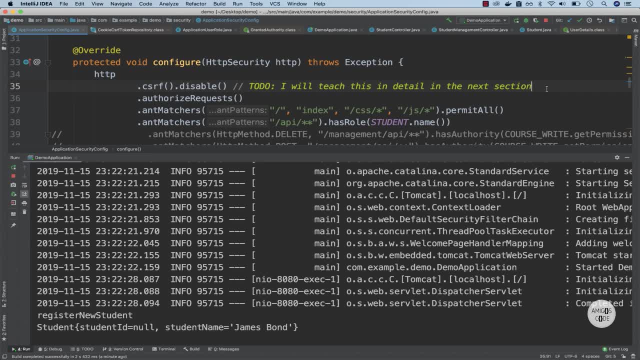 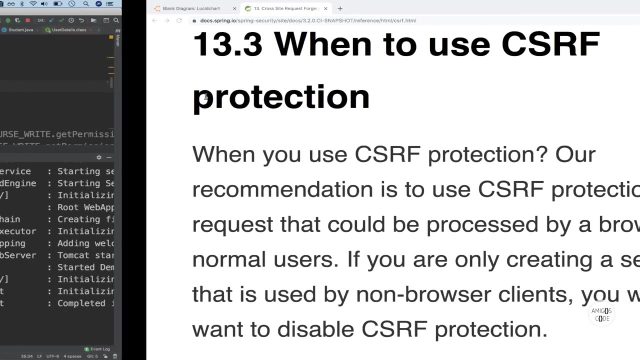 Done with this line right here. So in fact, I can comment this or actually remove this to do, because we are learning about this. So next let's go ahead and learn exactly how to send the actual token. So this token, right here. 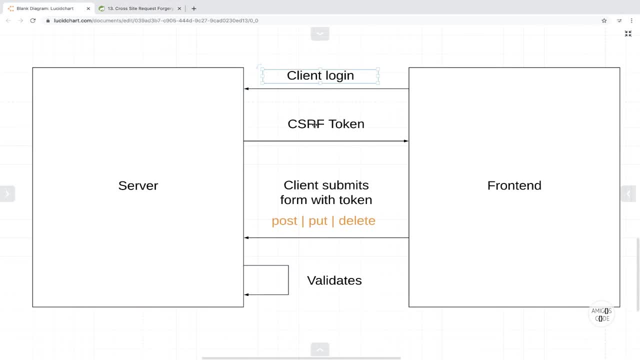 So right here. So when the client logs in, how do we see this token right here so that the client can use it to send it back Back to our server? All right, let's go ahead and learn how to generate this token to our 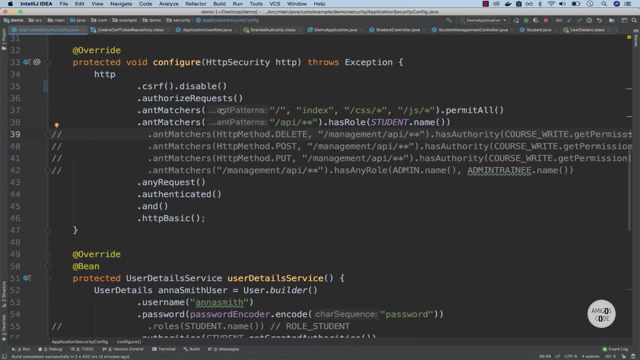 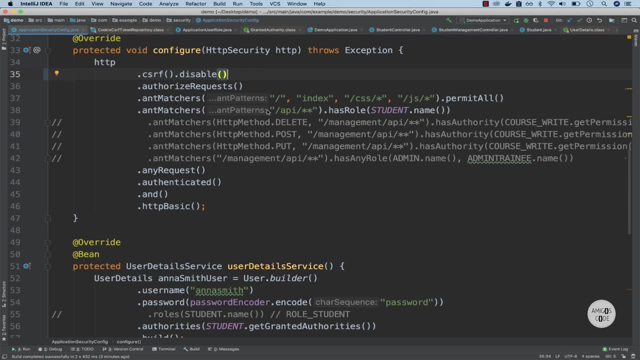 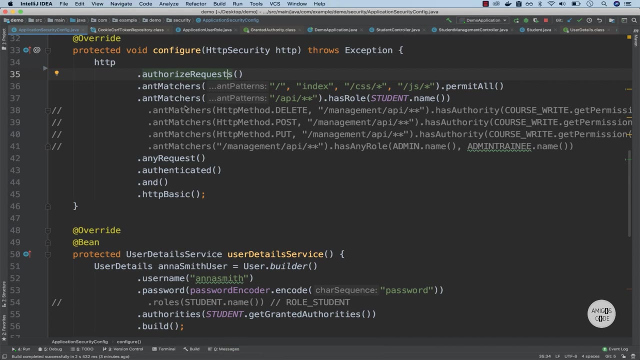 front end. So what we need to do first is to actually enable cross site request forgery. So, right here, what I want to do for now is simply delete this line. We're going to add it because we need to configure this, But for now, just go ahead and delete that line, because I want to show. 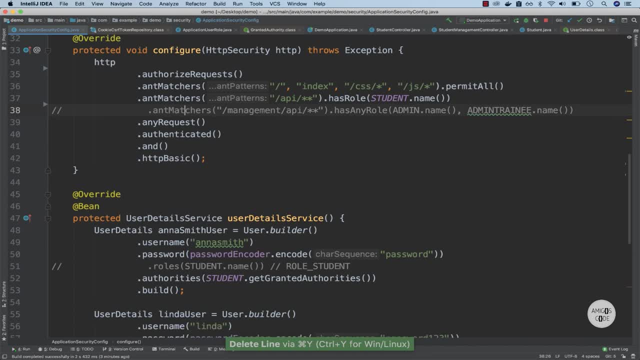 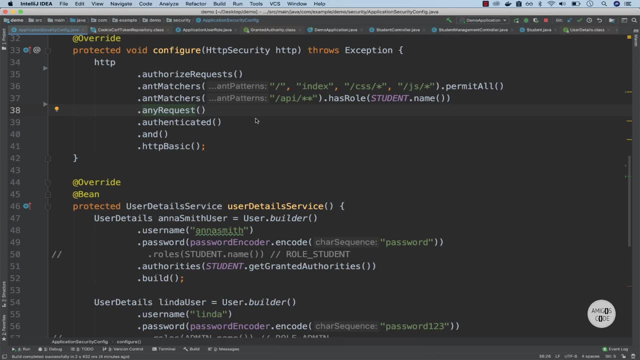 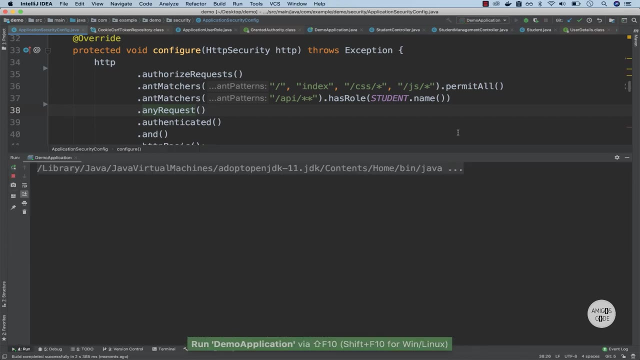 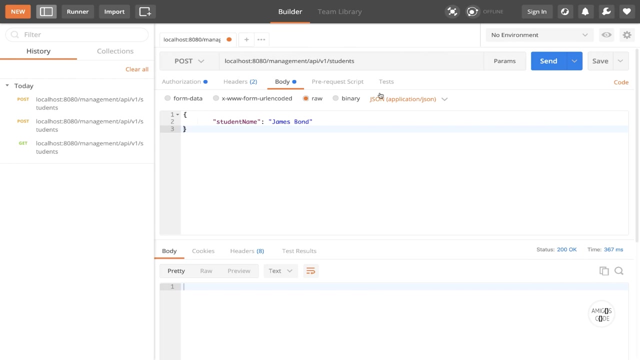 you something first, And also let's go ahead and delete all of these and matches, because we are using annotations And you can also get the source code from the previous branch. Now go ahead and restart the server and go to Postman And right here, let's go ahead and send a get request. 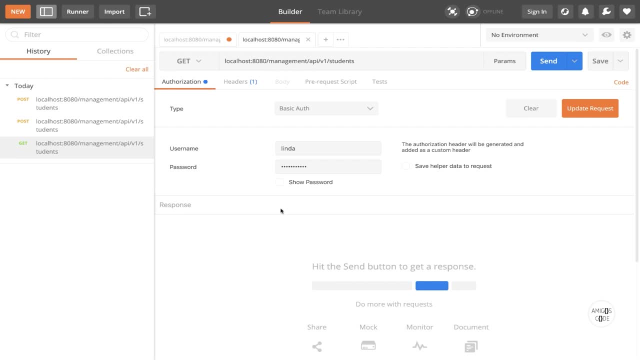 So, Linda, she's accessing management API and you can see the password is password 123.. Okay, Now let me go ahead and send this request, And you can see that we have 200 status code. So this is fine. So if you are using Postman, like me, go ahead and click on this. 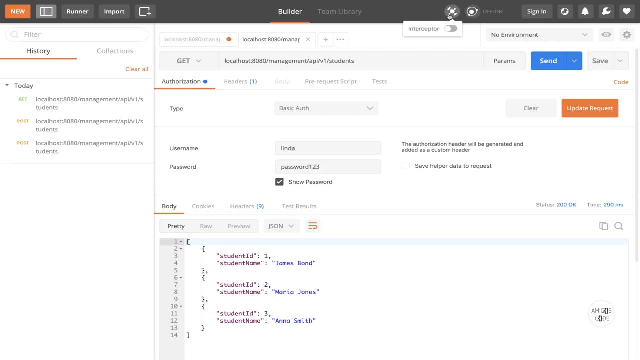 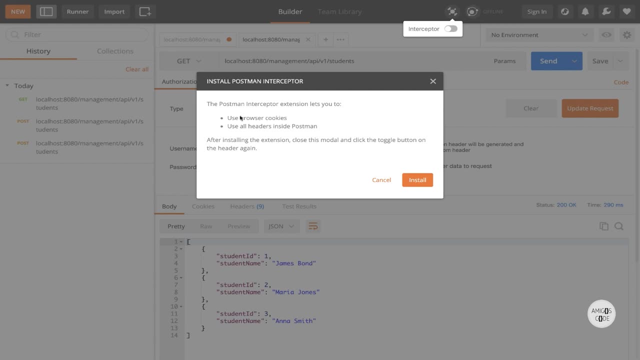 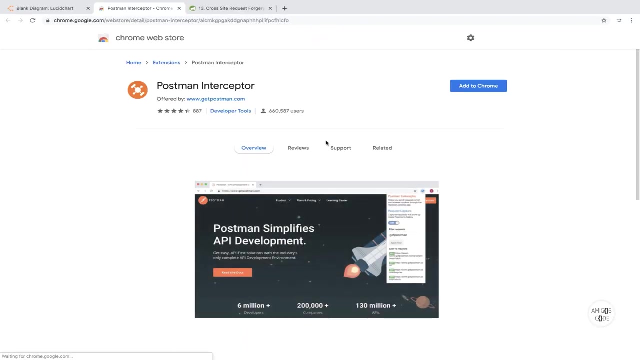 icon, which is the Postman interceptor. So I want to click on it and then simply enable And basically this allows us to use browser cookies and use all headers inside of Postman. So let me go ahead and install And I want to add it to Chrome. 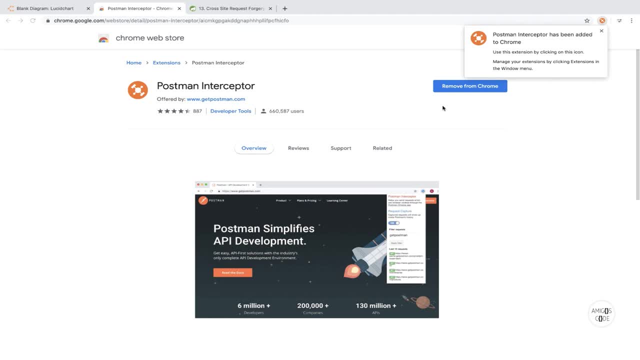 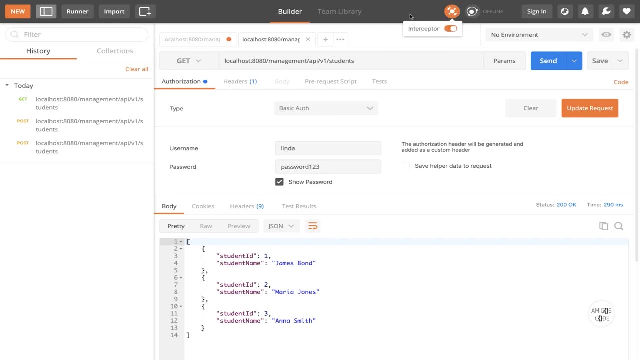 There we go. Now, if I go back, I think it should have installed: There we go. So this is now installed. So if I send the request again and then go to cookies, you can see that now we have some cookies. So let me actually remove it. 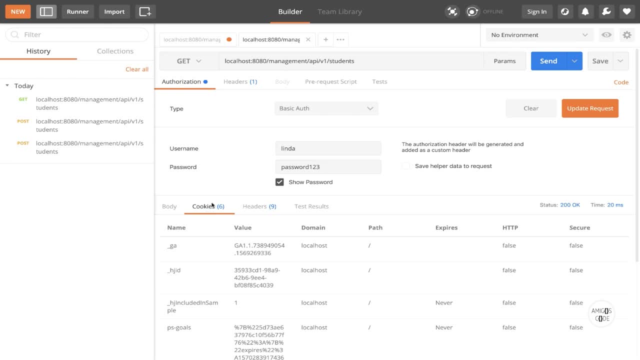 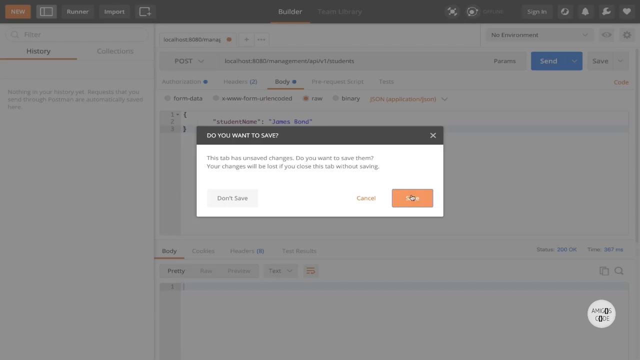 So send Oops. I think what we need to do is actually: let me clear everything. So let me clear those requests and this one as well. So I just want you to see exactly what I'm doing. So let me clear everything. So don't save. 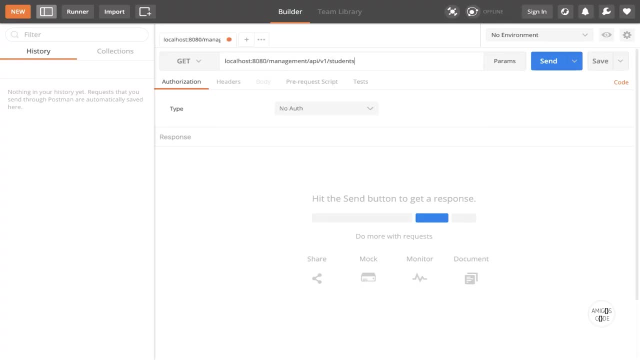 And this will be local host and then management. And if I send, you can see that we have zero cookies. Right, But as soon as we enable this interceptor. and now let's go ahead and send the same request. Now we have some cookies and I'm going to grab the actual token. 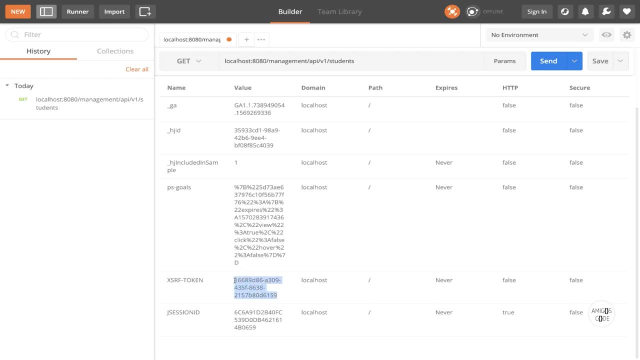 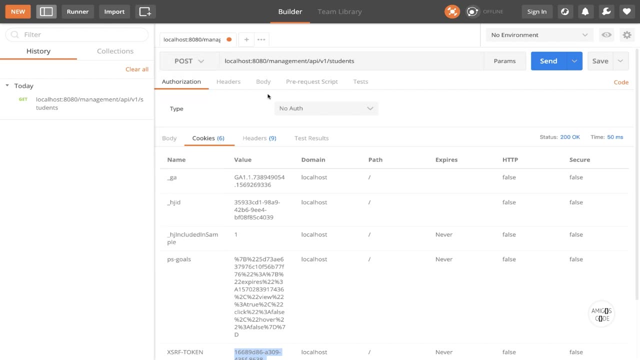 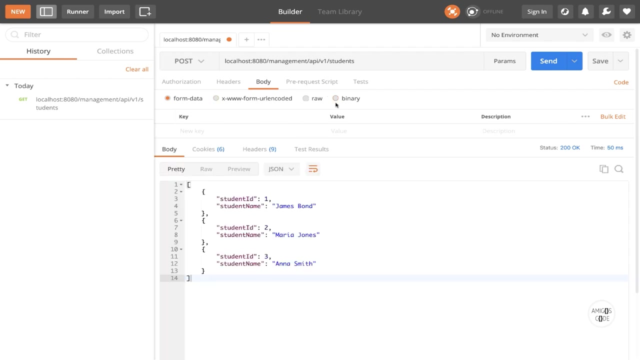 right here. So this is a token. So I want to press command C and then now let's go ahead and send a post request, So post, and then in the actual body, So right here. So let me scroll up. So in the actual body, right here, go ahead and just say: raw. 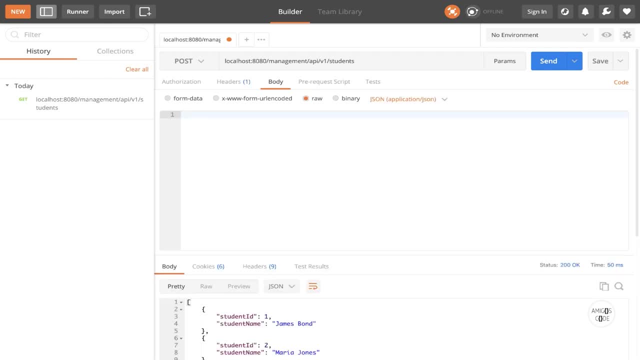 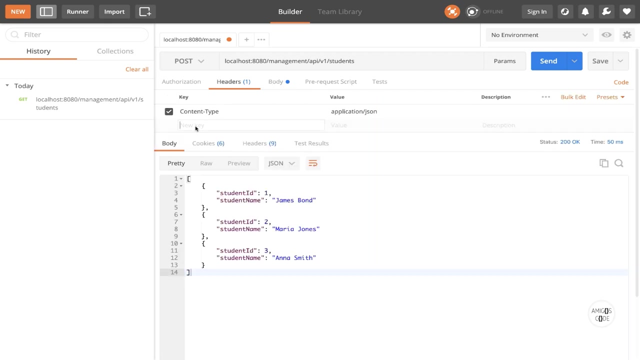 And then this will be JSON And right here student and the name and Alex and Gomez. And now go ahead and navigate to headers and go ahead and add the following: So X, actually all caps, So X, and then dash, XSRF, dash, and then token. 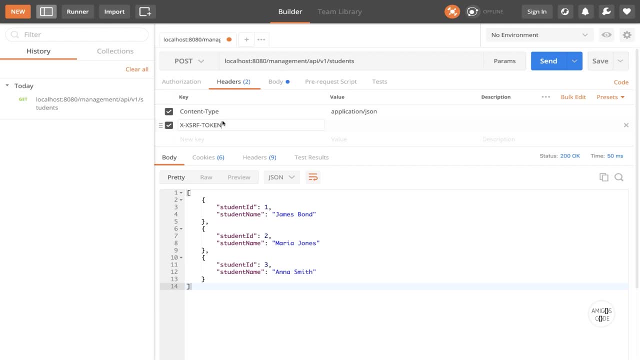 Okay, DASH XSRF-TOKEN. So this is the actual header that spring security is expecting. So actually, let me go ahead and just send this request as is. So if I send the request, you can see that we get forbidden. 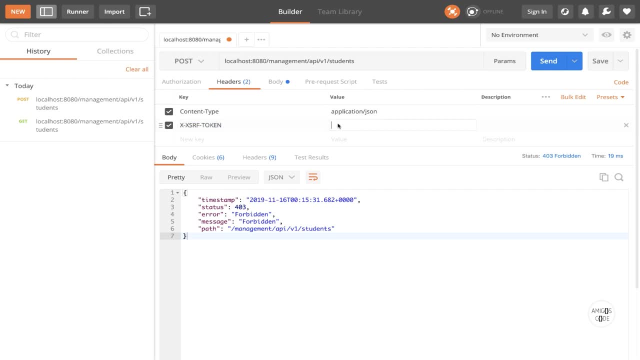 Now if I add the header and then paste the actual token, So this was a token, And now if I send, you can see that we have a 200.. And this is cross site request forgery with spring security. So obviously we are passing the actual token right here within postman. 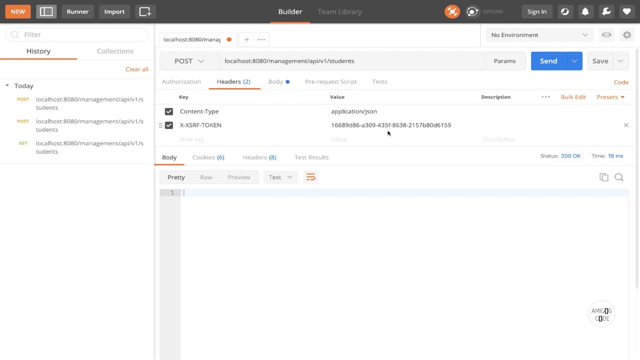 But this: for example, if you are using a react or angular, you need to implement the logic to get the actual token from the header, as we did right here. So remember, if I send the get request and then cookies, you can see that you can grab. 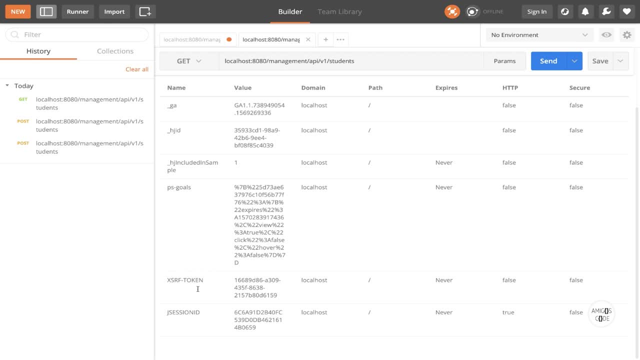 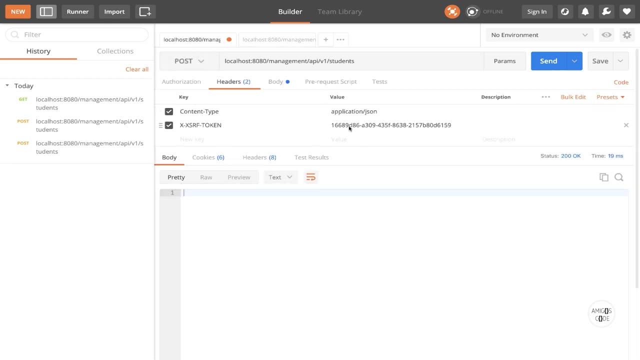 the header. So XS RF token, And then, when you perform the actual post request, you simply pass it, and then you pass the actual token. Next, let's go ahead and learn how this token is actually generated within spring security. All right, let's go ahead and learn how these tokens are generated. 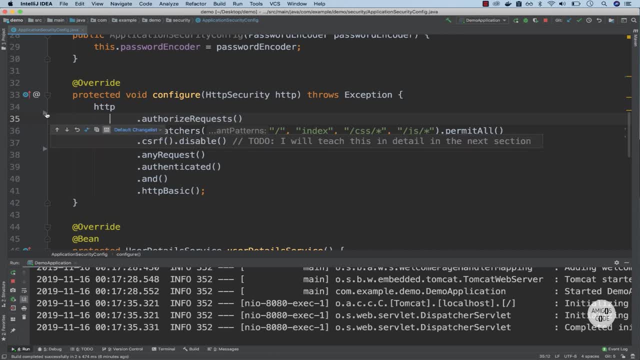 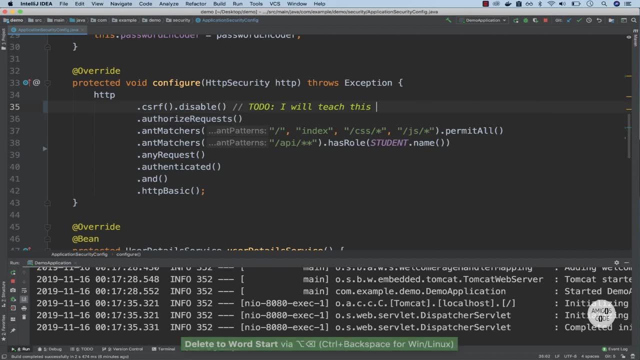 So let's go back to IntelliJ and right here let me actually revert the cross site request forgery I'm going to disable And now what I'm going to do is actually remove that and we're going to configure it. So, with cross site request forgery, there is a method called CSRF token repository. 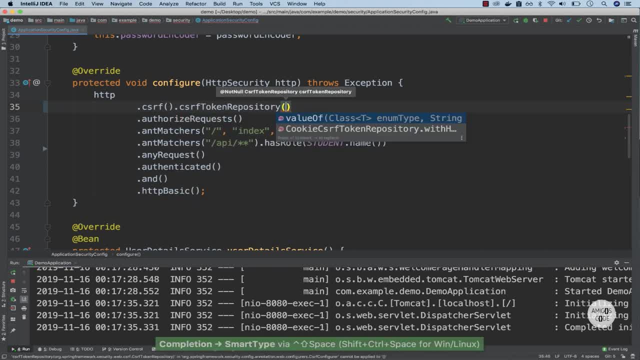 So go ahead and select it. And then inside, I'm going to say cookies: CSRF token repository with HTTP only false. And then, right here, I'm going to say cookies. And then, right here, I'm going to say dot and then end. 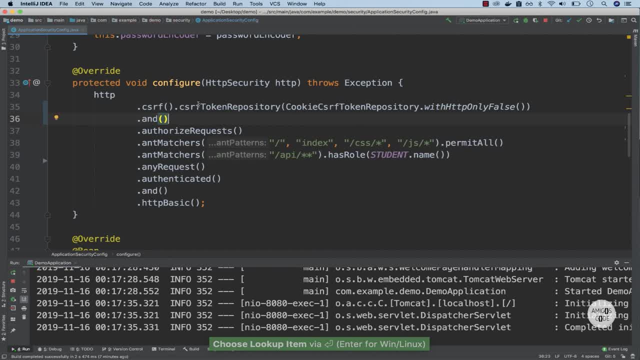 So right here, this is simply configuring how we are. So right here, this is simply setting up the actual repository, So how the tokens are generated. So, by default, spring security is doing that for us, but we can add some extra settings. 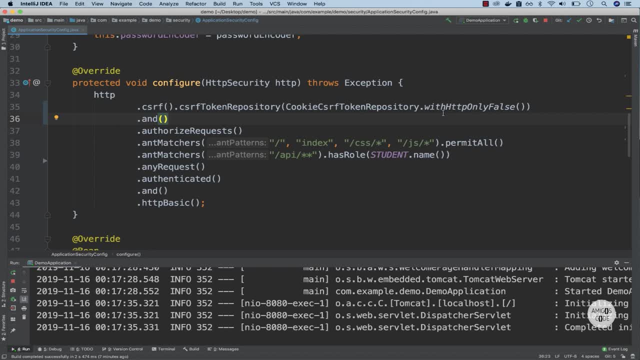 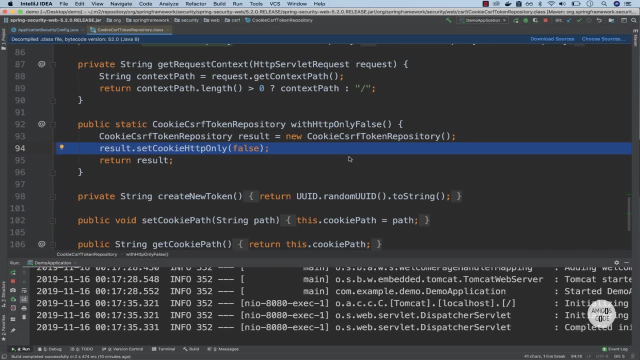 So right here you can see that we are passing with HTTP only false. So what This line right here means? it means that the cookie will be inaccessible to client side scripts. So if the client tries to access the cookies with some JavaScript, then it won't be able. 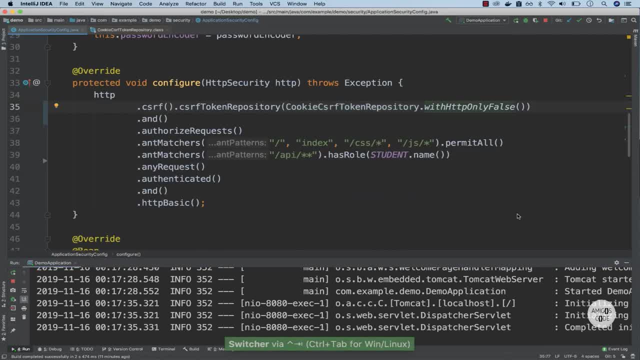 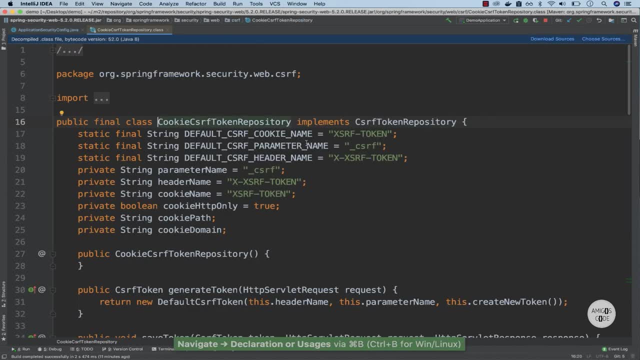 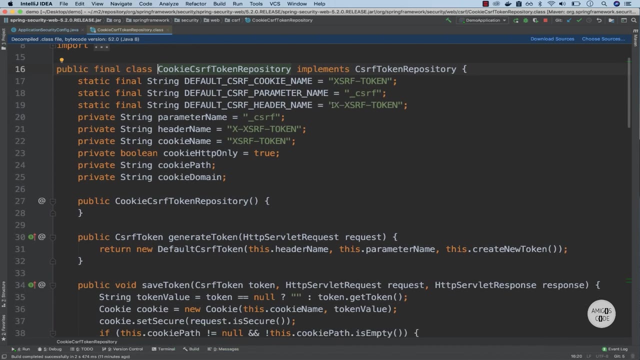 to do so Now. if I go back, let me just go back and let me collapse this. So go ahead and click on cookies: CRF token repository And I just wanted to see the actual implementation. So, right here, If I scroll down and you can see that this is the actual header, 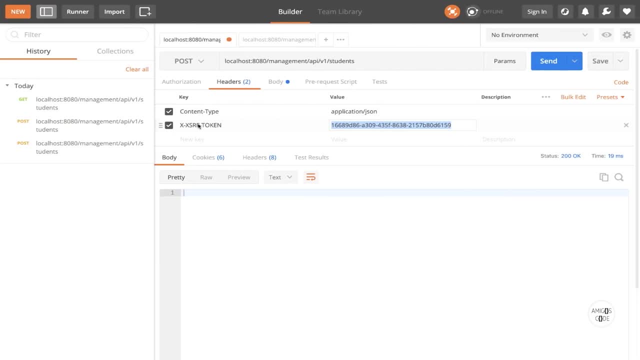 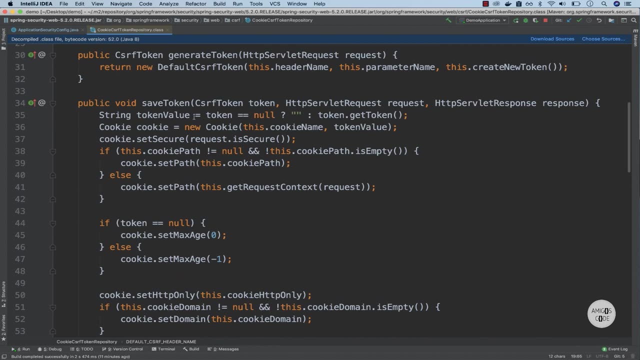 So this is what we have defined right here. So this is the actual header, remember. So right here, if I scroll down, you can see that you have a safe token right, which generates a brand new token and then creates a cookie, sets the security and then sets the path. 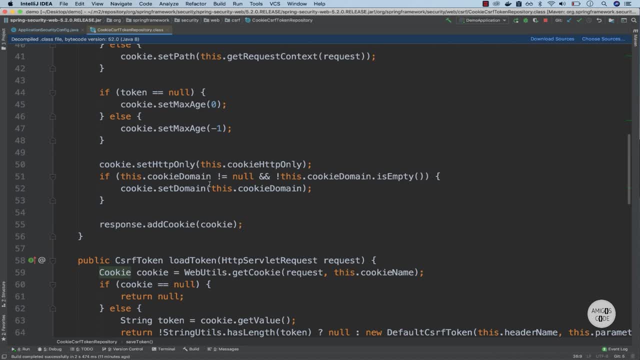 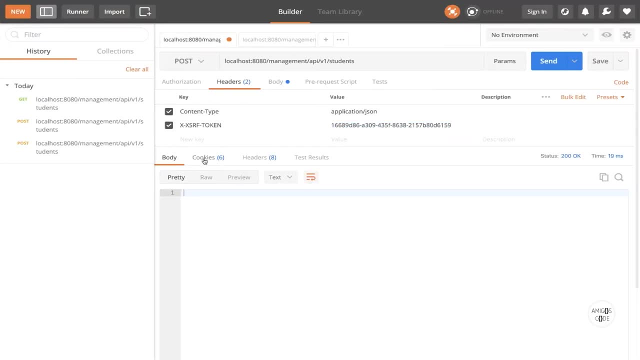 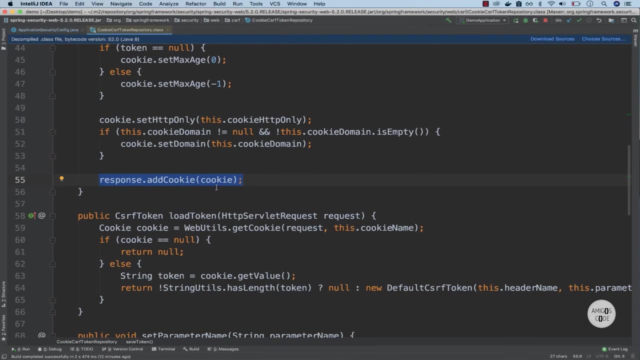 And you can see that it's setting like the max age And right here it simply adds a cookie to the actual response right. So this is this bit right here. So we are getting the actual cookie right here because of this implementation. 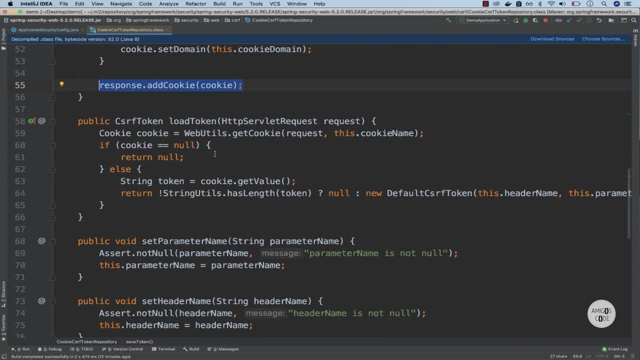 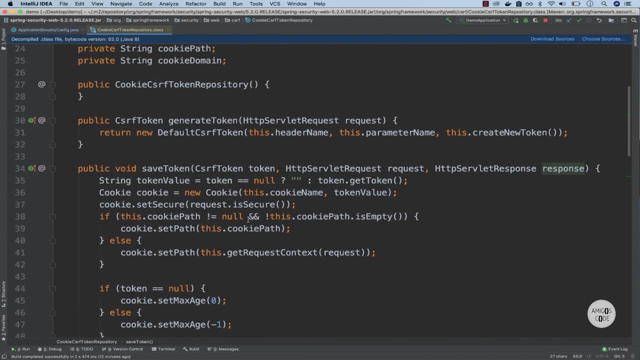 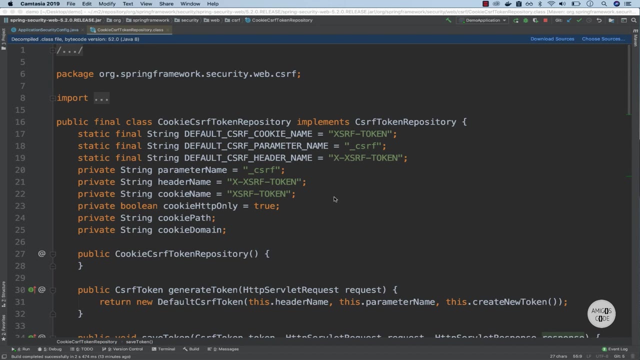 The same with load token: It loads the cookie, if there is any, And you've got some other methods right here. So, basically, go ahead and read this class to get a full understanding of How this works. And finally, another class that I want to show you is this one: 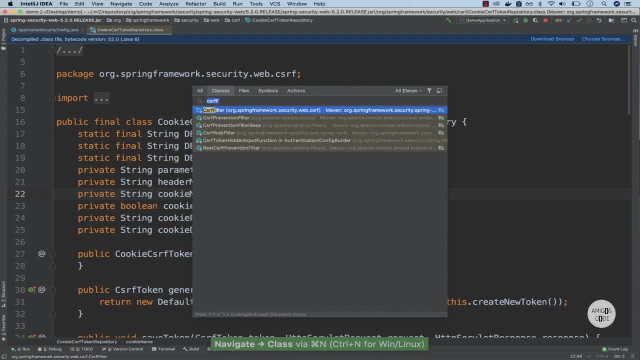 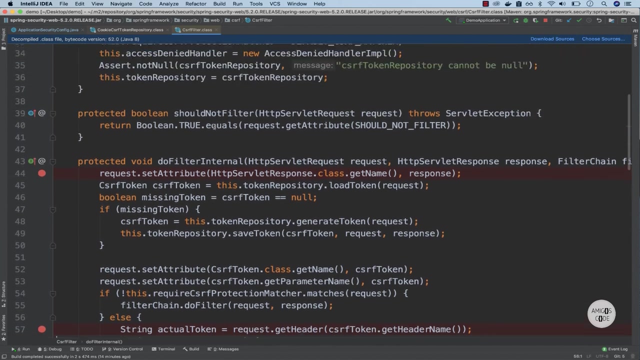 So go ahead and press command N and then search for CSRF and then filter. So this one from spring framework security, So the very first one. So go ahead and click on it And basically, right here, So this class, right here it's a filter that runs. 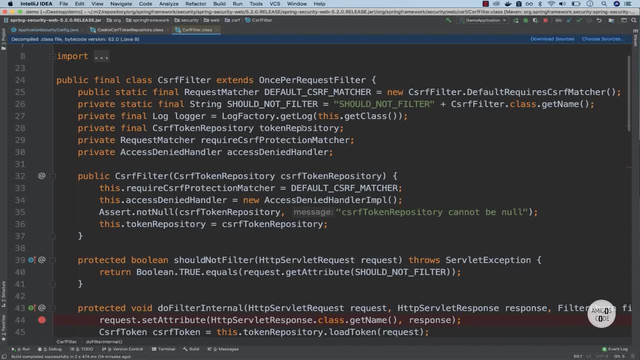 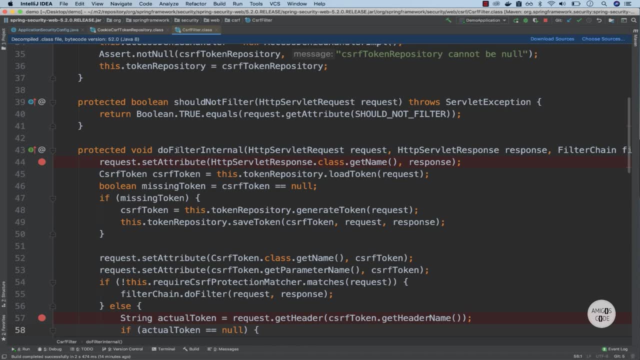 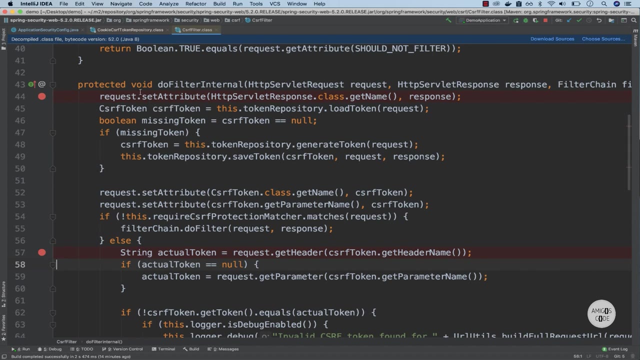 So if I scroll up it runs once per request. So basically you can see that there is this filter called do filter internally, And right here you can see that the implementation is very simple. So it set some attributes, Then it tries to grab the token, right. 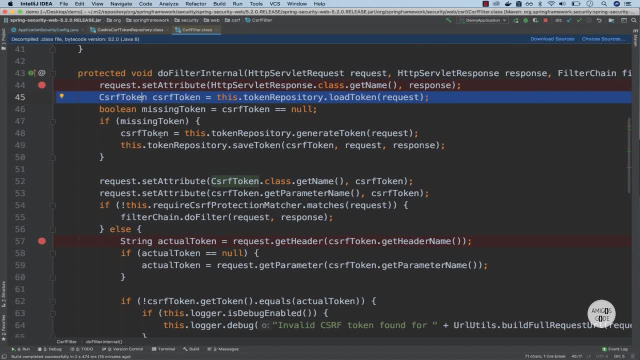 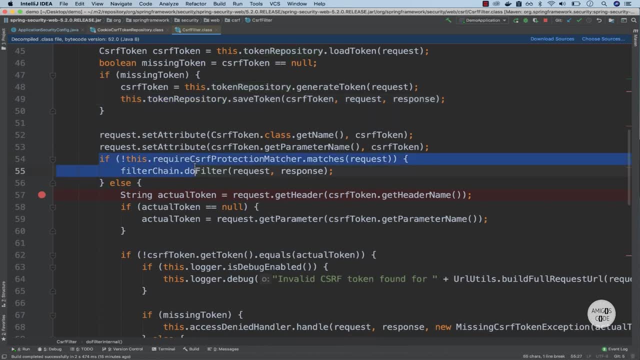 So this is grabbing the token And then, if it's missing, it generates a brand new token and then saves it to the repository And then, right here, it checks whether we need to actually check the token based on the request, ie if the request is a post. 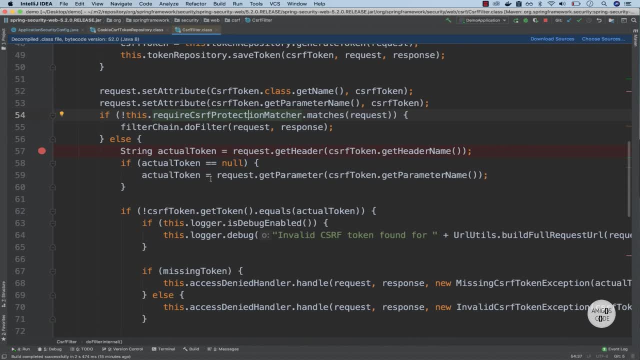 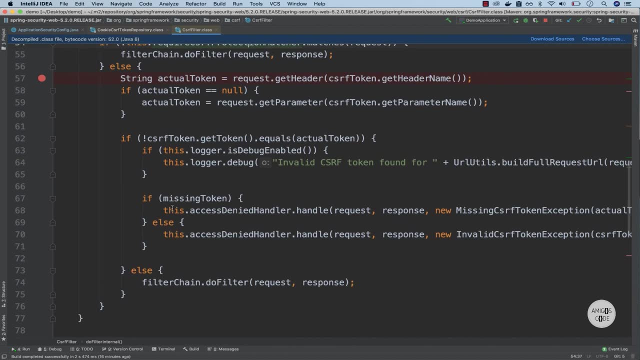 put or delete. If so, then we actually try to get the actual token right here And then we compare the tokens Right And then right here you can see that if the token is missing we get access denied, And also if the tokens are not the same, you can see that. 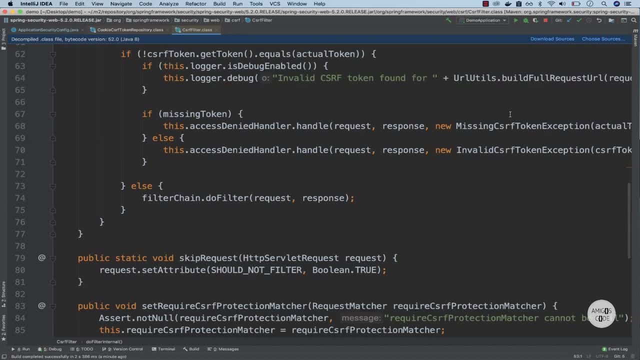 we have invalid token found And this is all for this video, So if you have any questions, go ahead and drop me a message. Otherwise, let's move on. All right, By now you should know how the cross site request filter works, Right. 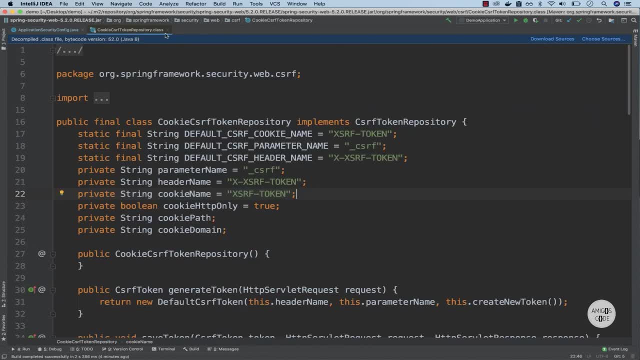 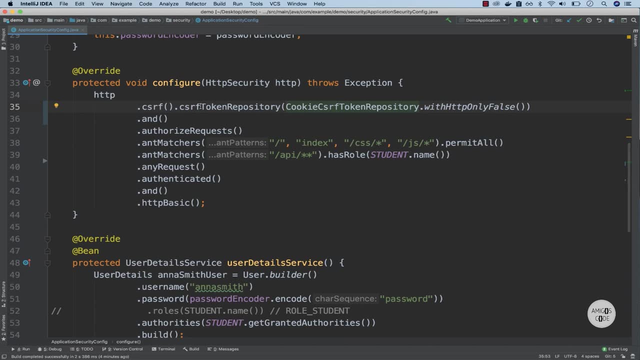 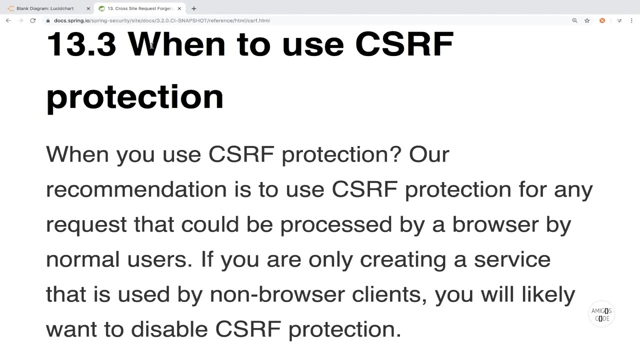 And also how the token repository is implemented. So I think that now you have a clear understanding of what is cross site request forgery, And also you should know when to use it, Right, Right, So let me actually remind you. so the recommendation: 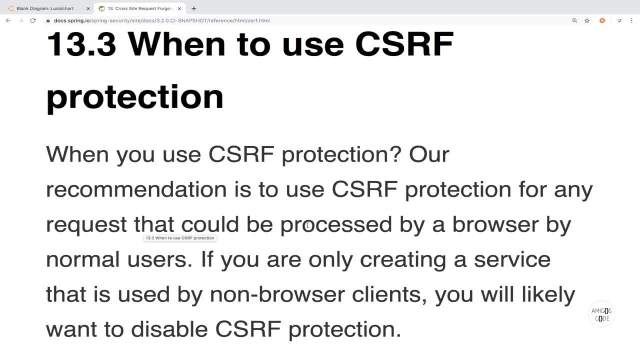 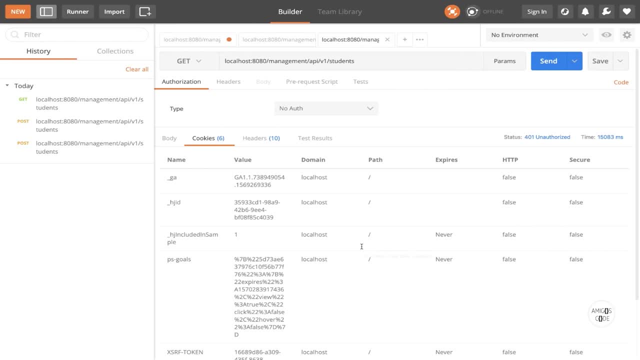 is to use this protection for any request that could be processed by a browser, by normal users. If you are only creating a service that is used by non browsers clients, then you likely want to disable it, And that's what I'm going to do, because I'm using